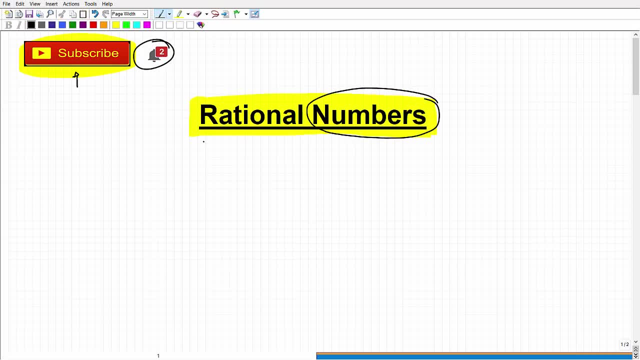 Here. it's important that you understand this in order to really have a grasp on rational numbers. So, basically, when you're in elementary school, middle school and like the beginning of high school, until you get into more complex math, you really focus on learning and mastering what we call the real number system, right? So this is a basic real number line, So let's just write that down: real 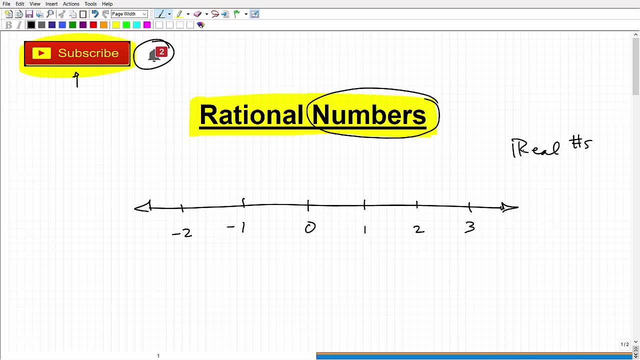 numbers. Okay now you might say: well, what are the numbers? are there? Well, as you progress, more like saying algebra two, you know, if you're taking more advanced math and you're finishing up in high school, or definitely in college, you're going to be learning complex numbers. Okay. so there's other, more complicated number systems that you know you'll be learning above and beyond the real numbers. But real numbers is what you really have to master and understand: rational numbers. 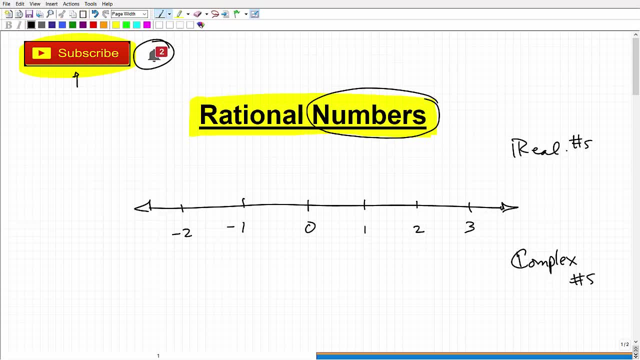 Okay so the real number system is all the number types on a number line. Okay So, in contrast to complex numbers- complex numbers you won't be able to plot on a number line like this. Okay so, real numbers: you have 0123, negative one I go to. you're probably familiar with these numbers as being integers. Okay so these guys here are integer numbers. 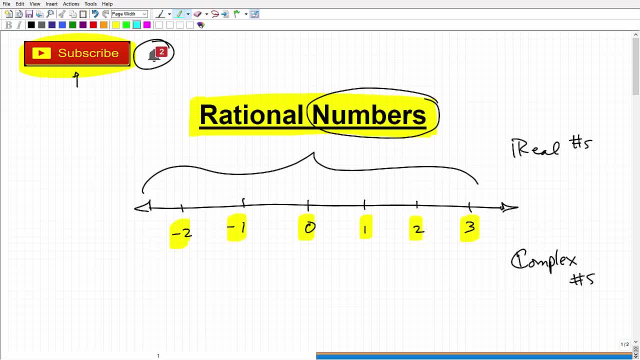 Okay, then you have. if I just talk about 123 here, I could define these guys as the counting numbers, natural number system. if I throw on a zero, I have the whole number system, etc. So the real numbers. okay, have all these different subsets of type of numbers on them. Okay, so let's just quickly. 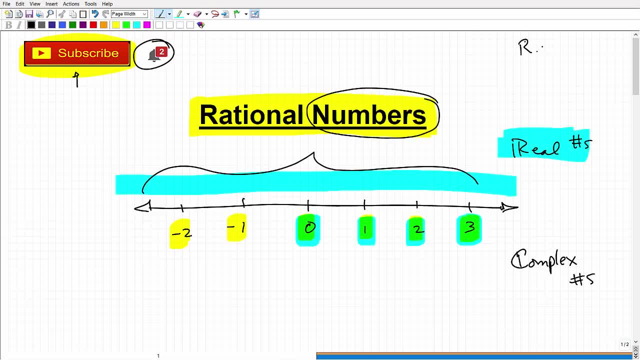 review them. Okay, so on the real numbers, real numbers system, you'll have like the counting numbers- sometimes it's called a natural number system- whole numbers. you'll have integers and then you have Q. Okay, now, Q is a rational number. So let's go ahead and define rational number now And then actually just let's put it up here, just so we don't forget: I are irrational numbers, So numbers are either rational or irrational. Okay, when we use this word, 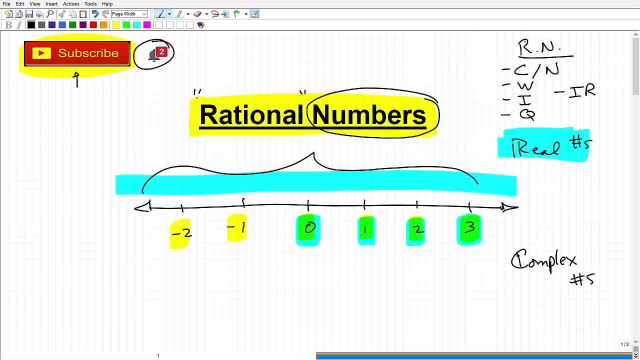 rational. okay. so what does this mean? Let's give you the big definition Now. basically, a rational number is a number that you can write as a fraction. Okay, Now, it's not just any fraction, it's a fraction using integers. Okay, So any number you can construct, turn into a fraction is a rational number. So one half is a rational number, negative three. 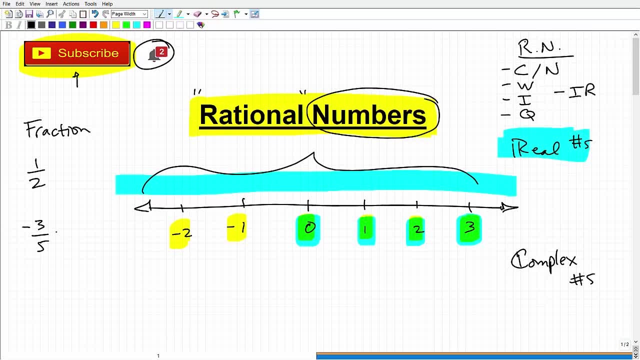 fifths is a rational number. Okay, even let's say two, now two. sometimes these numbers can have more, be classified and in a lot of different ways. So two is a natural number or a counting number, It's also a whole number, It's also an integer And it's also a rational number, because two you can write as two over one. So any number you can write as a fraction, where the numerator and denominator 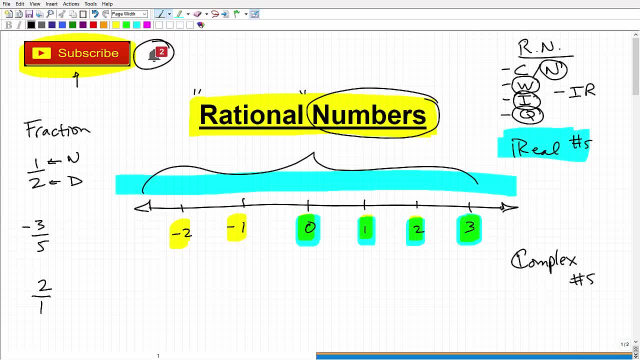 are integers is a rational number. Now let's take a look at kind of stealthy rational numbers. What if I said 0.25, is that a rational number? So you know a lot of students say no, that's not. 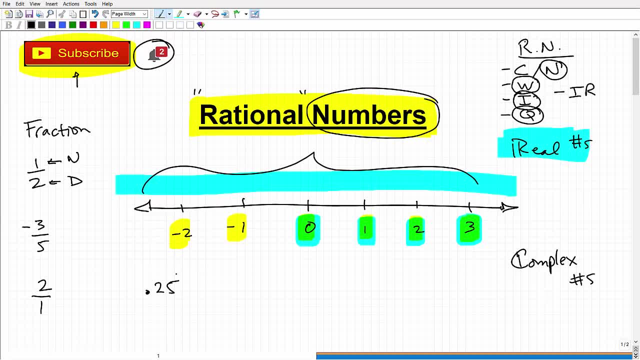 a rational number. That's not a fraction. That's not what I said, right? What I said was, if you can write the number- okay, as I did too- as a fraction of integers, that's a rational number. So 0.25 is equal to the fraction one-fourth, okay. So therefore it is a rational number. 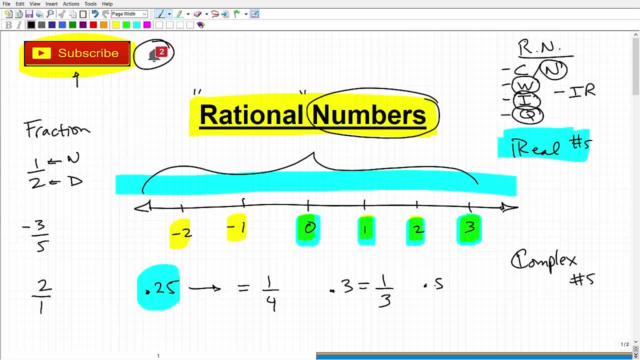 0.3 is the fraction one-third. 0.5 is the fraction one-half, right, So all these decimal decimals here are in fact rational numbers. Now let's go ahead and contrast this to an irrational number, because it's important that you understand that, And I think we'll kind of 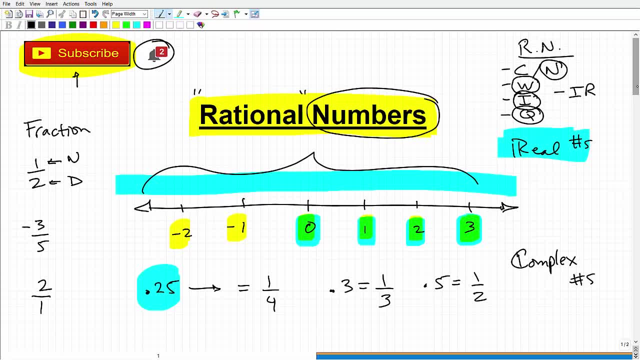 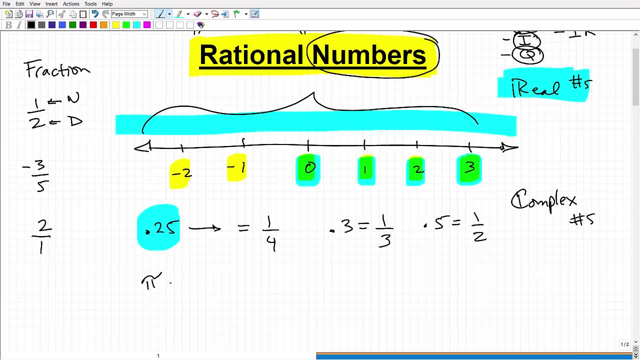 wrap up the video so we don't make it too long. So an irrational number is a number that you cannot- you cannot write as a fraction. A good example of this is the number pi. okay, Or well, most of you probably know that that's around 3.14.. Now that number. 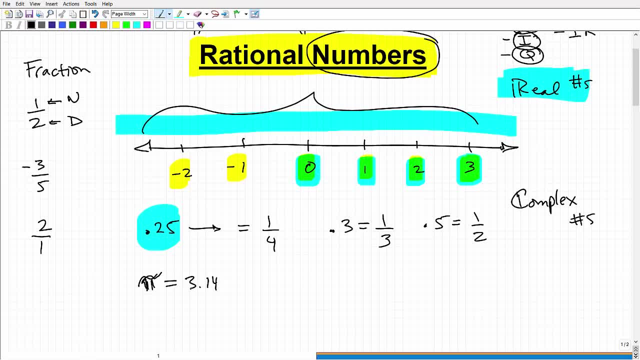 is not equivalent to 3.14.. That's just a estimation. The deal with pi, okay, the reason why we have this symbol, because this number goes on and on and on. I don't have a calculator in front of me so I don't know the digits off the top of my head beyond 3.14,. 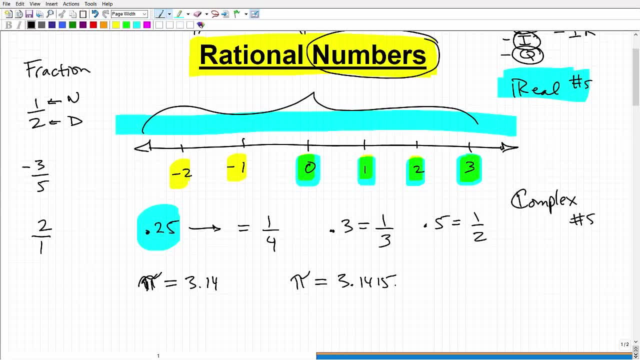 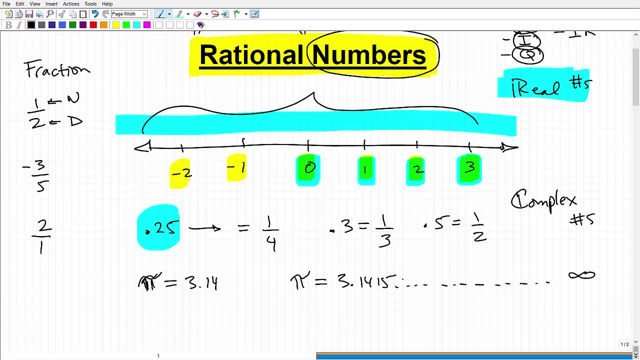 non-repeating. okay, So the digits are not repeating. So in other words, if I have three point, for example, if I have 3.1717171717, you can, this is a repeating decimal. So if I have, 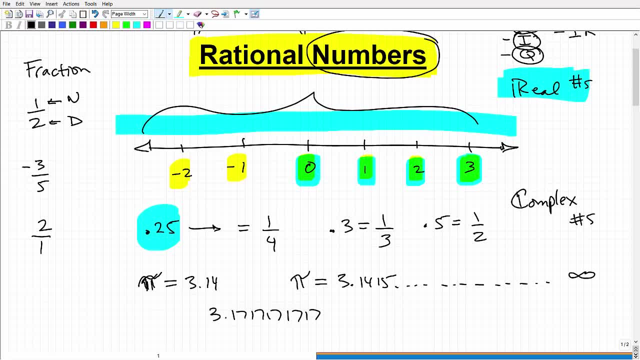 three point. for example, if I have 3.171717171717,, you can. this is a repeating decimal. Okay, Oftentimes you can rewrite these as a rational number, Matter of fact, you can, but that's for. 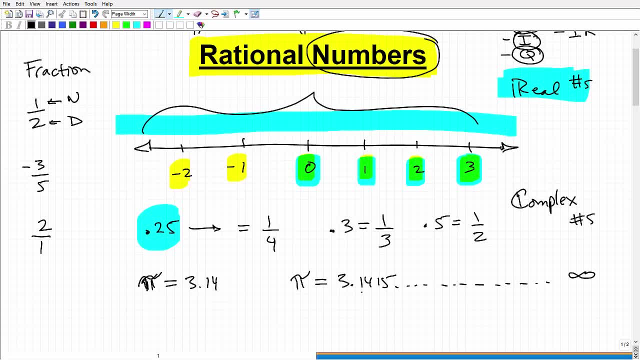 another video. The deal with the irrational number is it's non-repeating. okay, So the digits here are just coming up random: 2,, 7, I mean it's nobody's guess, you actually have to know. So it's non-repeat, it's not repeating in any particular manner and it's non-terminating. 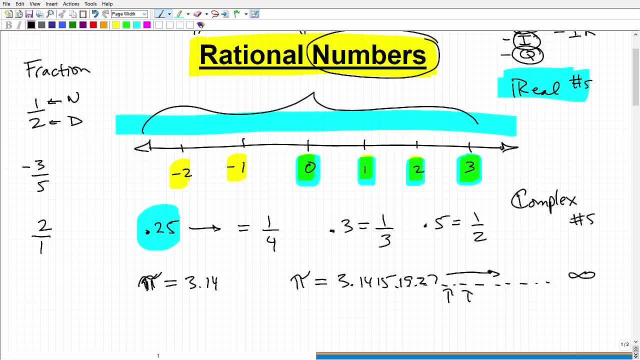 So it just goes on forever, with random digits coming, etc. So instead of trying to write this entire number out, which is impossible, we just give it a symbol. okay, Pi. So other examples of irrational number would be like, say, square root of 2, okay, The square root of 2 is also an irrational number. okay, If you look. 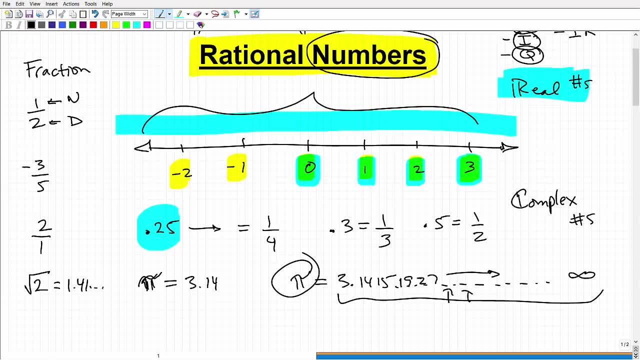 in your calculator you're going to get a decimal: 1.141, da-da-da-da. Just because the decimal stops on your calculator screen doesn't mean it terminates. It keeps going forever in a non-repeating, non-terminating fashion. So when we're looking at decimals, we're trying. 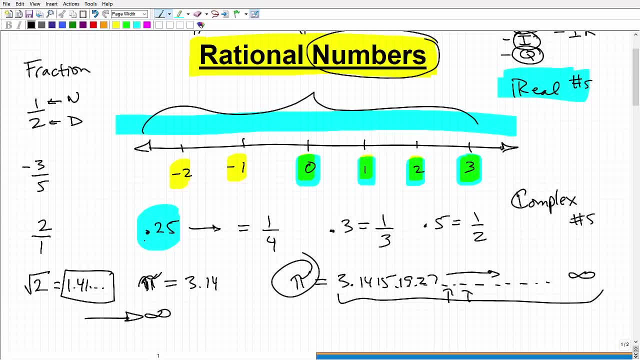 to identify what a rational number is. Remember, a rational number is a decimal that you know has a pattern and it stops, okay, But really the most important thing is that you can take that decimal and write it as a fraction. So these are some basic examples here of that. 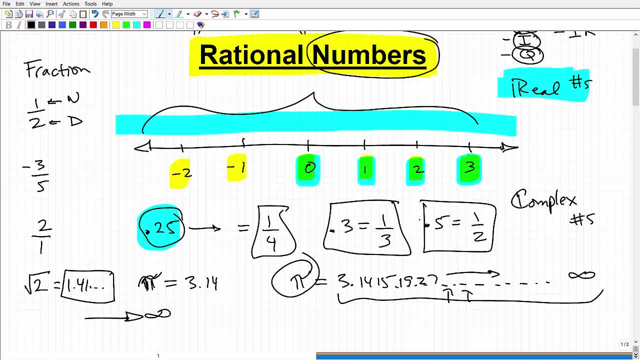 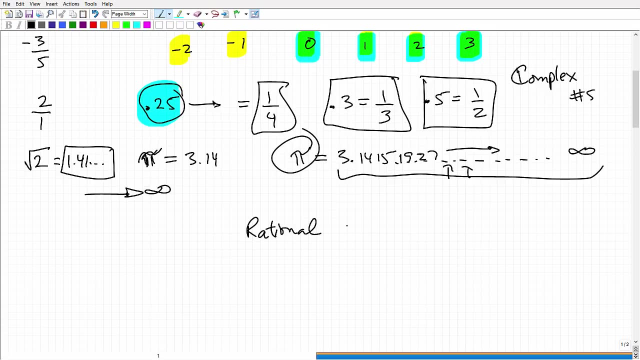 So wrap it up: A rational number is a number you can write as a fraction, where the numerator and denominator are integer values. But I'm going to give you one little bonus definition here, and that is rational expressions. Rational expressions, So in algebra we have rational numbers right. So like we had, say, two-fifths is a rational. 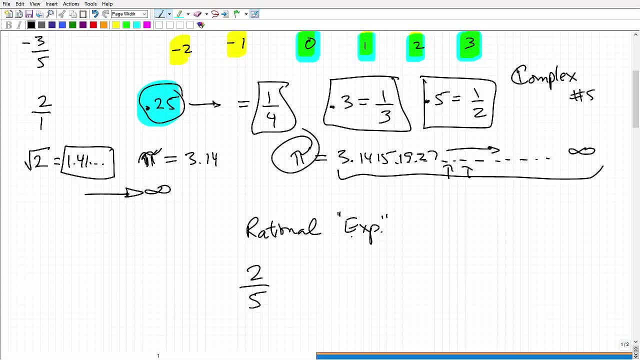 number. But when we use the word expression and not number, now we're talking about basically a fraction that involves variables. So if I have 2x plus 1 over x, now I'm dealing with a rational expression. okay, Not, this is a rational. 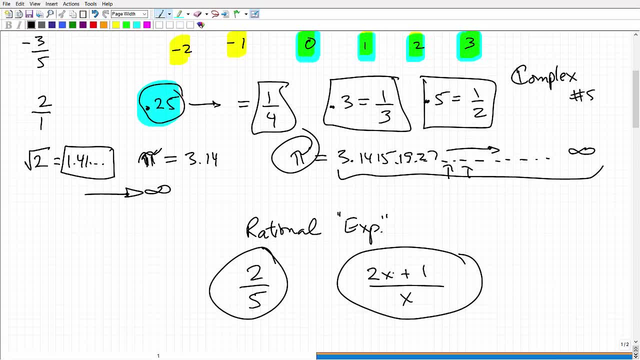 number. this is a rational expression, But basically the idea. when you hear rational, you really need to be thinking in terms of fractions. Rational expressions in algebra even have a little bit more specific definition, but essentially fractions okay, But not any fraction, One last. 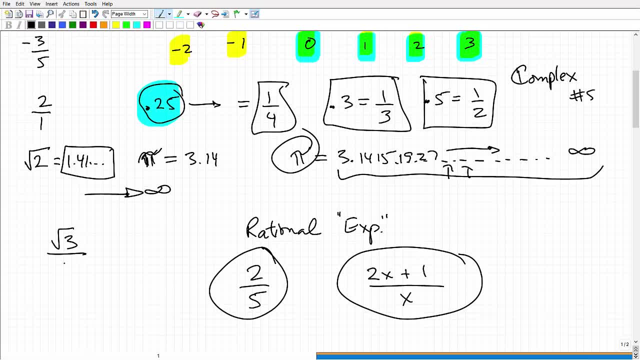 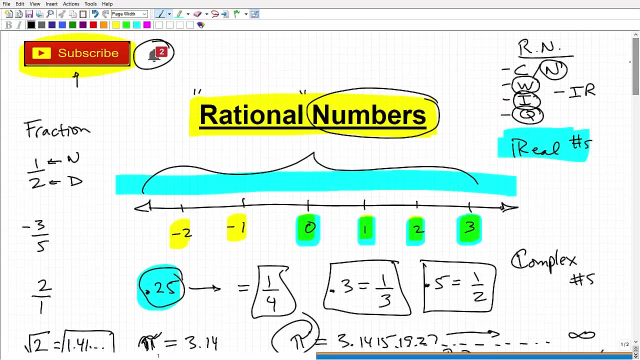 little check here of understanding. If I have the square root of 3 over 2,, this is not a rational number, because, although it's a fraction, don't be tricked. okay, This is not an integer. This is an irrational number. okay, All right, so let's wrap this up. That is rational. 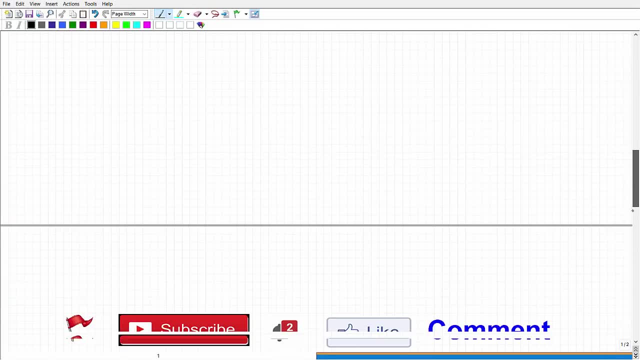 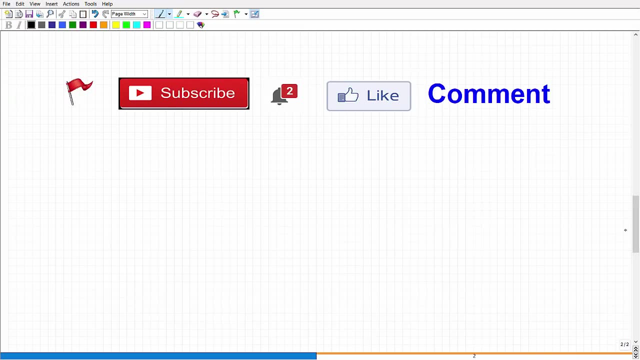 numbers. Hopefully you know I was able to explain this in a decent amount of time, but I didn't want to leave you, you know, without all the really important information. So, again, I hope you consider subscribing to my channel. You'll find tons of useful videos on various 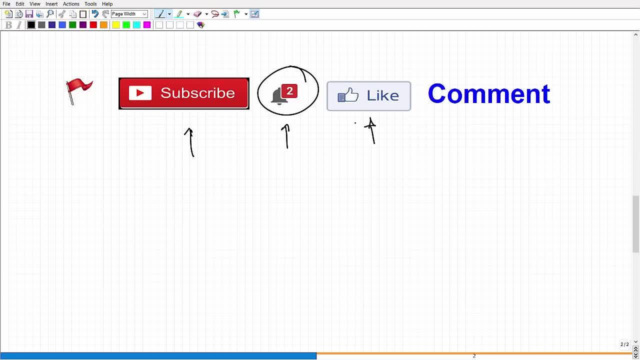 levels of mathematics. Make sure you hit that bell notification. If you got something out of this video, I'd definitely appreciate a thumbs up and leave me some feedback. It's kind of the way I know how I'm doing and if people have particular questions or want me to do a video, 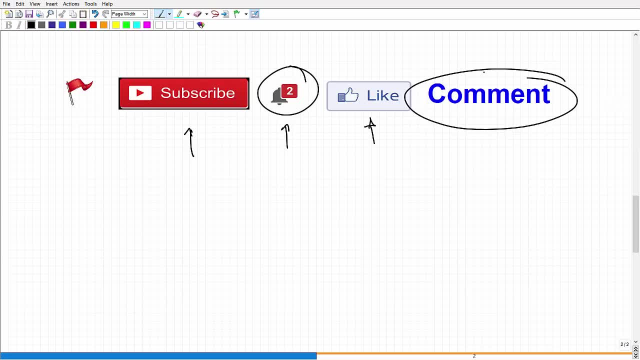 on a specific math topic or whatnot. I'm happy to do so. So it gives me ideas, it helps me improve. But, with that being said, I definitely wish you all the best and have a great day.